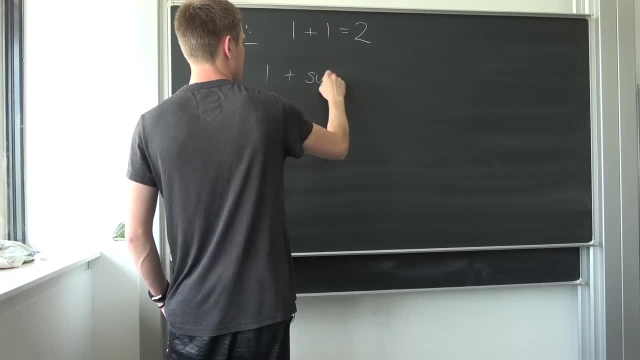 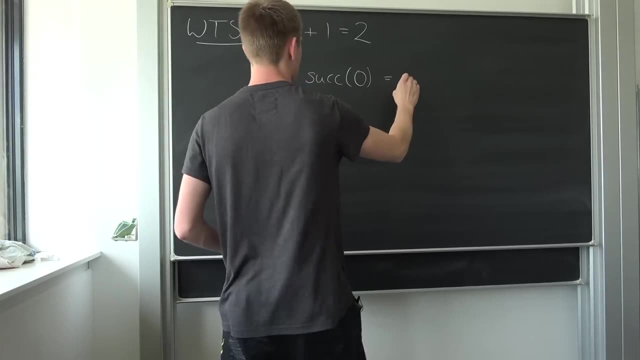 we have: 1 plus 1 is nothing but 1 plus the successor of 0, suc of 0. and well, we can use the second rule of addition on this one. So that's nothing but the successor of 1 plus 0. But by the Peano axioms and regular addition. 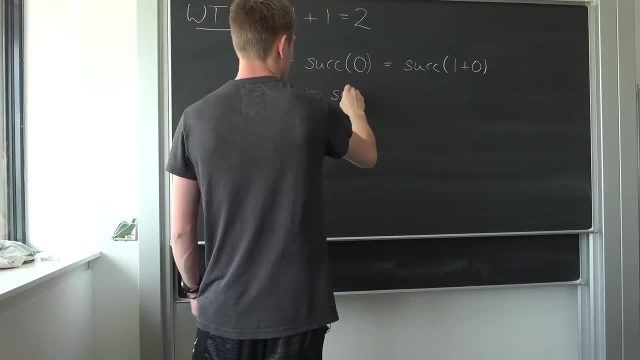 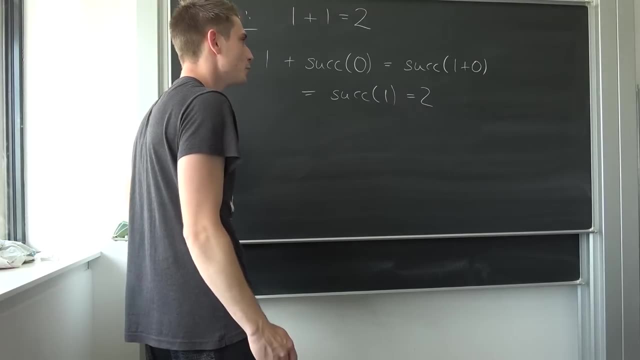 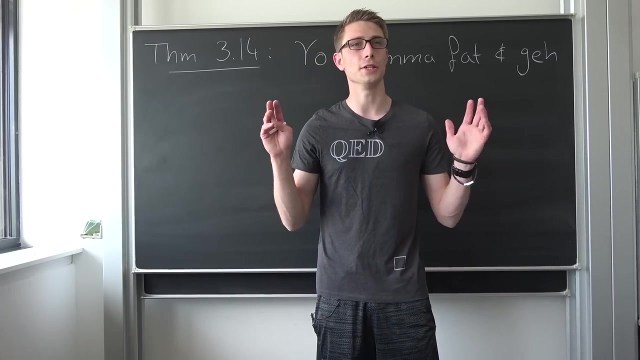 we also know that 1 plus 0 is nothing but 1.. So that makes the successor of 1 and by definition that's 2.. So that was easy. A direct proof really helps out here. This right here class is going to be the first proof by contradiction you are ever going to see. It's a real classic example. 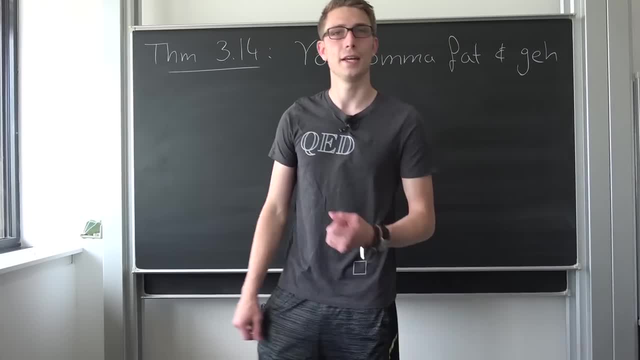 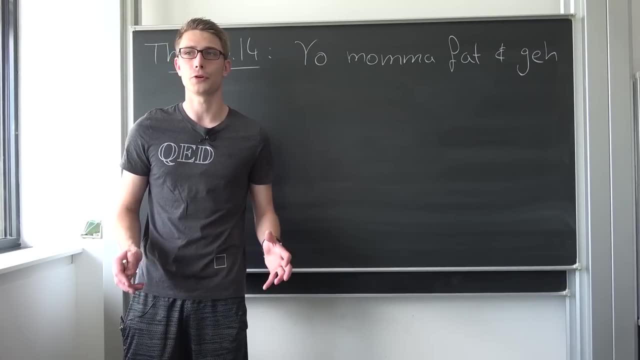 we are going to prove today Theorem 3.14 in the algebra course. Your mama, fat and gay. How can we prove this theorem? Well, why not strive for a contradiction? We are going to negate this statement and we are going to 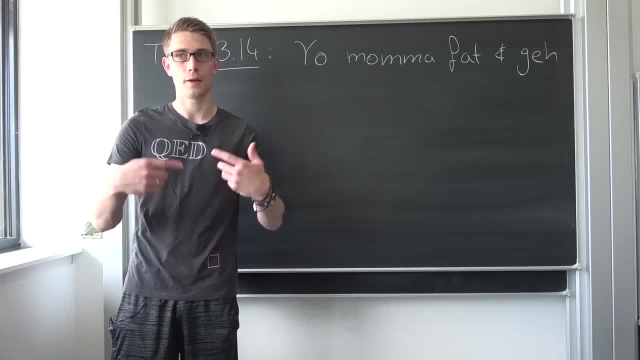 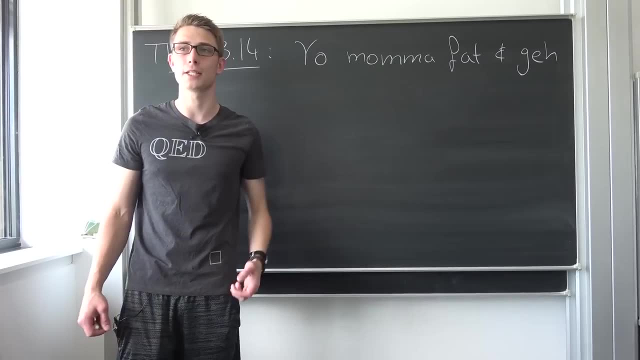 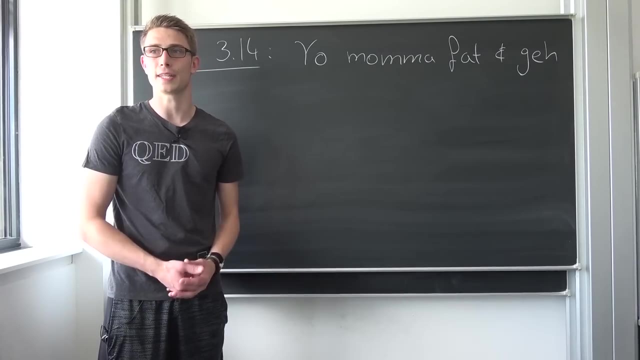 to show that the negated statement is wrong. This is what we call striving for contradiction and thus, by simple first-word logic, this original statement is going to be true. So why not negate a statement? The negation of your mama fat and gay is: your mama is not fat and gay. 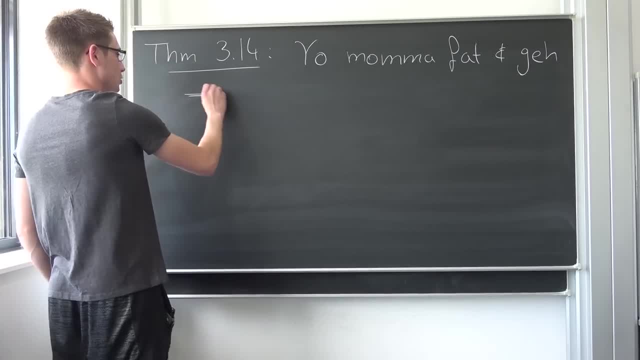 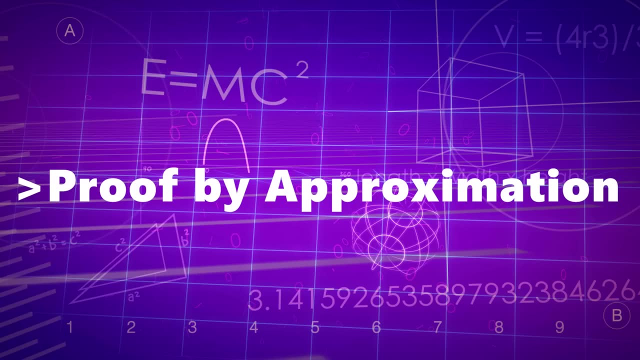 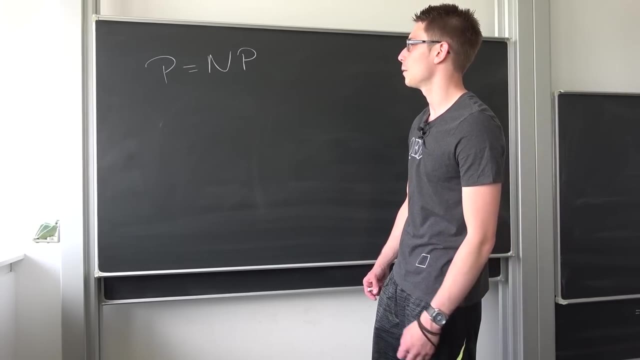 But that would be an absolute lie, meaning our theorem is indeed true. okay, I would say QED on this one. That was an easy example. Hey, Andrew, do you also want to have a coffee? P equals NP. You are still working on this stupid problem. 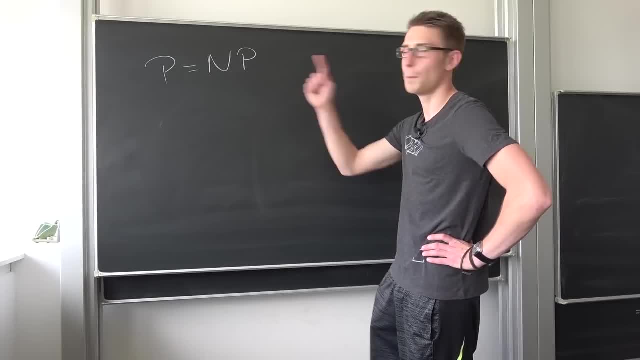 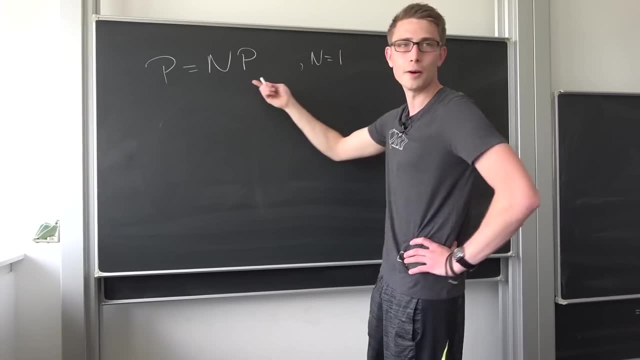 Seriously, Andrew, can't you see that you're basically for small values of n, really small values of n? Let's say n is equal to 1.. Well, this thing definitely holds. okay, P equals to P. I really don't know what the fuss is. 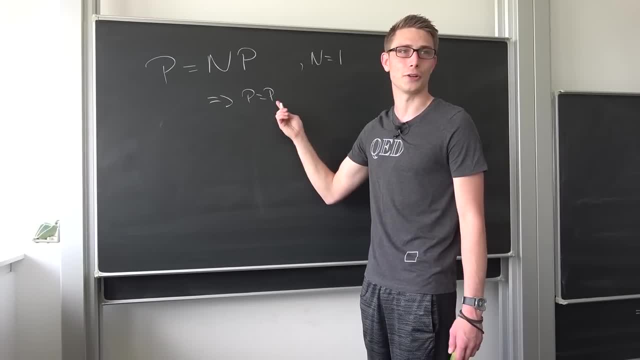 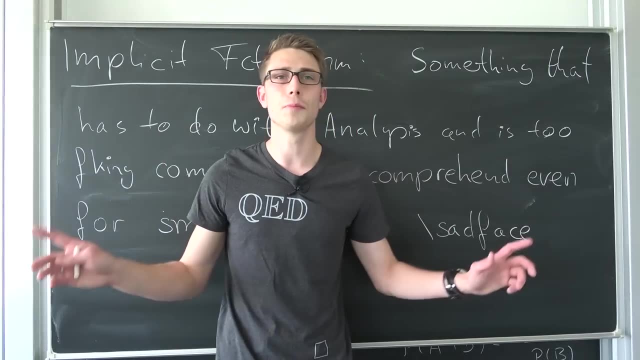 All about on this problem right here. Why the fuck are you going to get $1,000,000 for this triviality? oh goodness, Good morning class. Today's anal class is going to take quite a while, as always: one and a half hours. 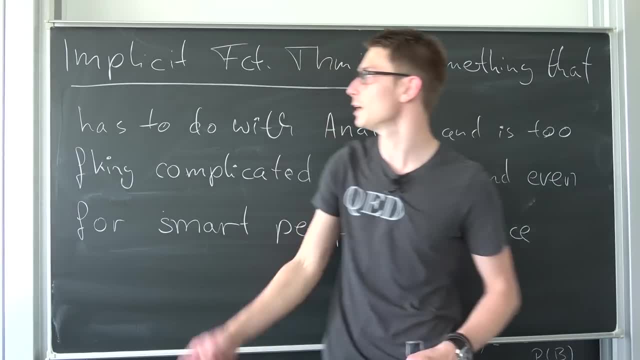 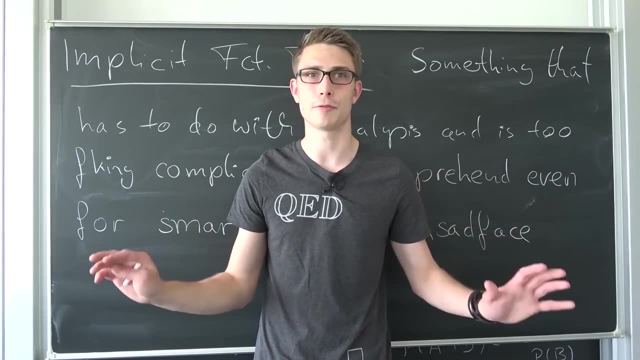 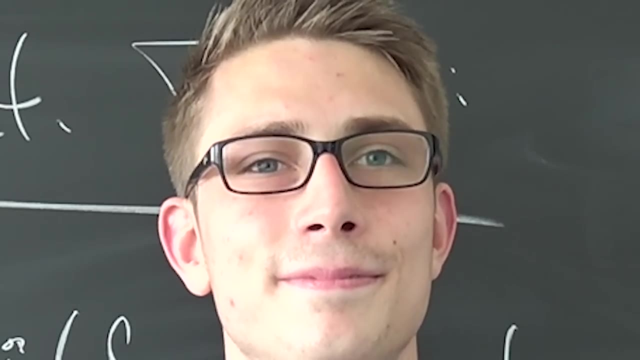 But today we only want to prove one theorem, namely the implicit function theorem. It's a very hard to prove theorem in analysis, so I hope you are prepared for over an hour of analysis Analysis action right here. I hope no one's going to notice that I have no idea what I'm doing. 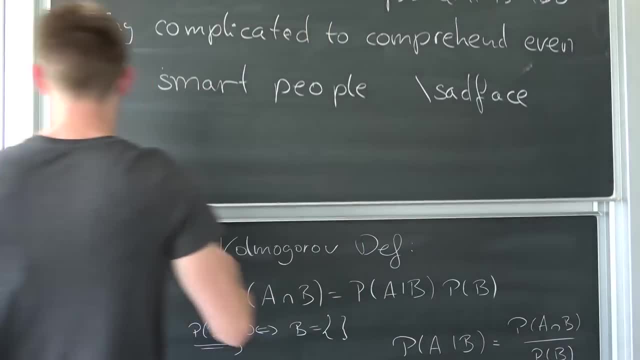 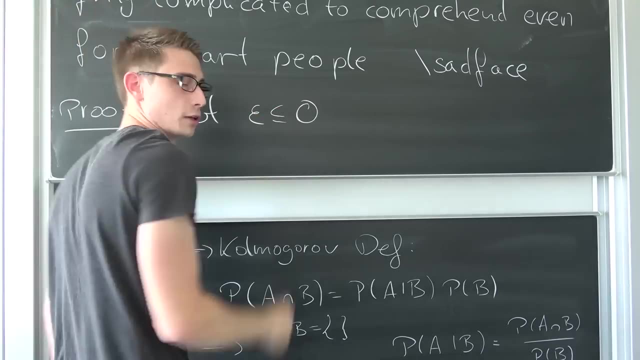 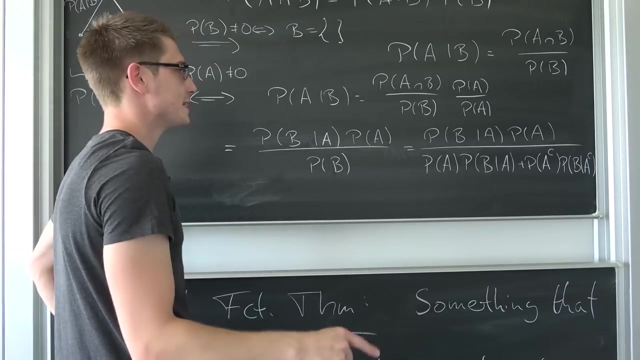 Let us start So. at first, I would like to assume that we have some epsilon being less or equal to 0. So all of this basically leaves us with some psi, Which is element of the complex numbers, And then we have some psi. 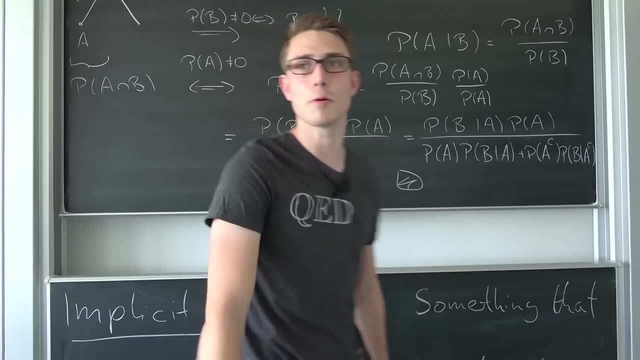 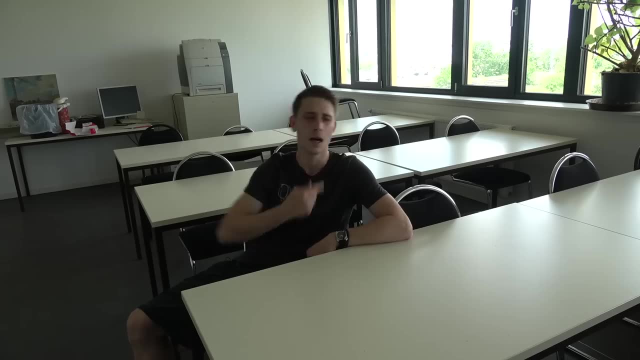 And with this we are done. I would say that was a huge success. This took quite a while and I hope everything was easy to understand. Excuse me, Mr Dodson? Yes, Andrew, I think you made a huge mistake. 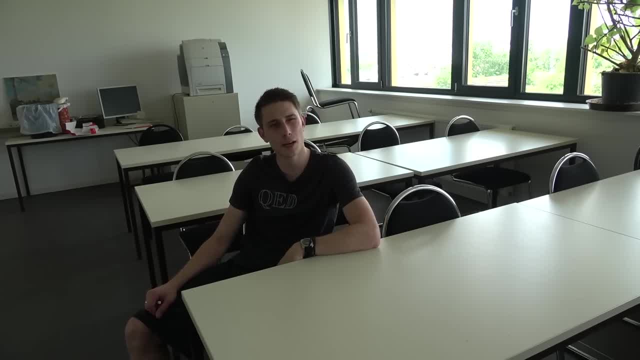 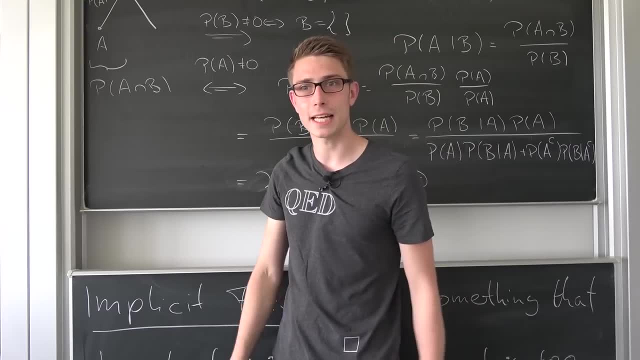 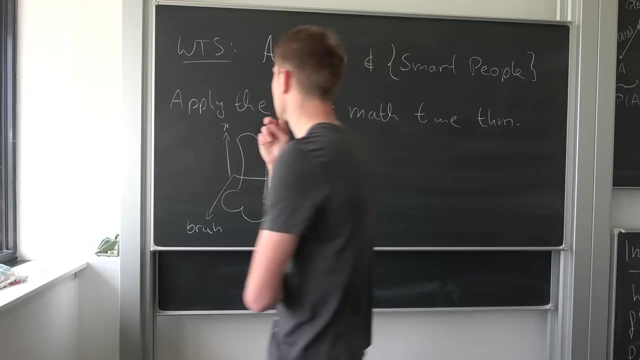 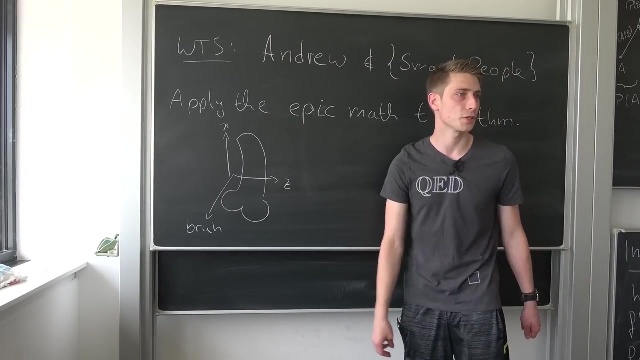 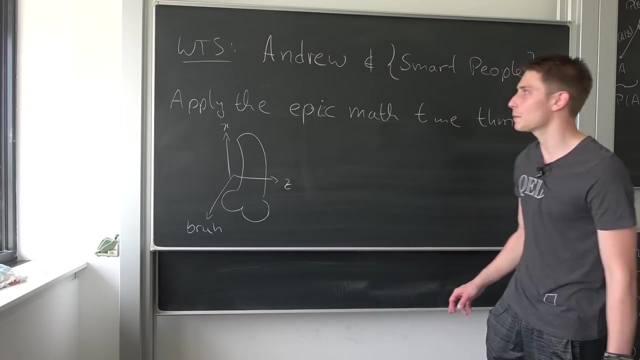 at the beginning of the very proof. Since when are we assuming that some epsilon is less or equal to zero? I said we are done. Andrew, Q-E-U-D Guys, this proof is going nowhere. Where should we even start? I mean, we tried applying the epic math time theorem. 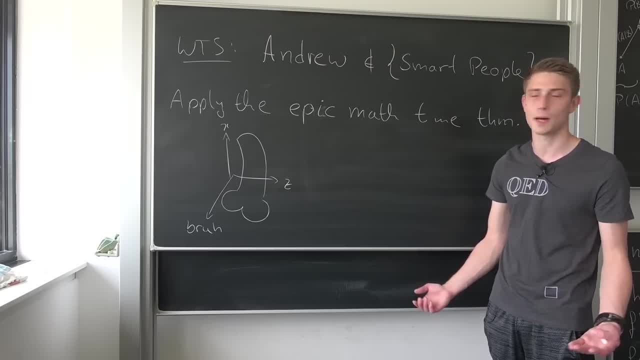 but we can't show that Andrew is not element of the smart people. I really don't know where to start. We even applied the big don't know where to start. big don't know where to start. But we have the wrong theorem down here. 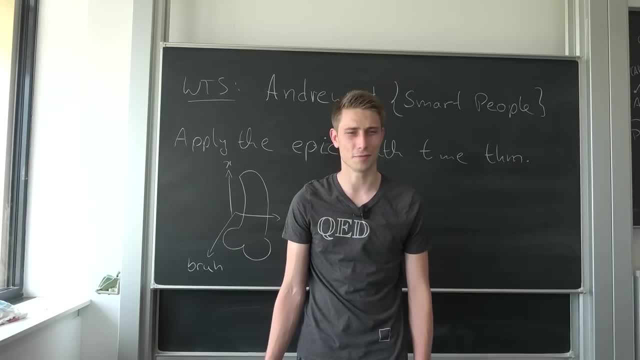 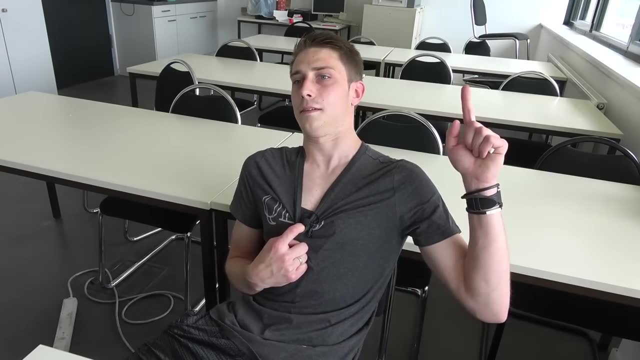 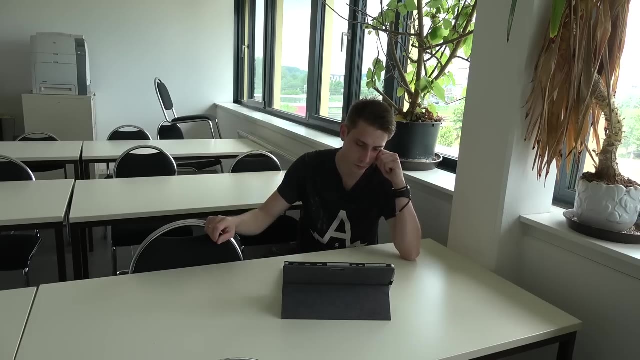 Should we just call it quits? Actually, Jonathan, that's a really good idea. Should we just stop? Please raise your arms? Yeah sure, Why not? Oh, yeah sure, I think we are done, then I consider this to be proven. 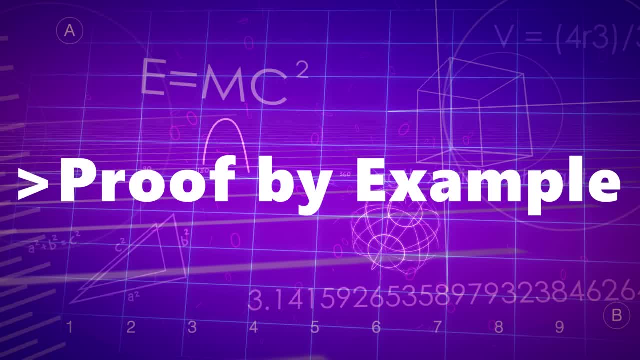 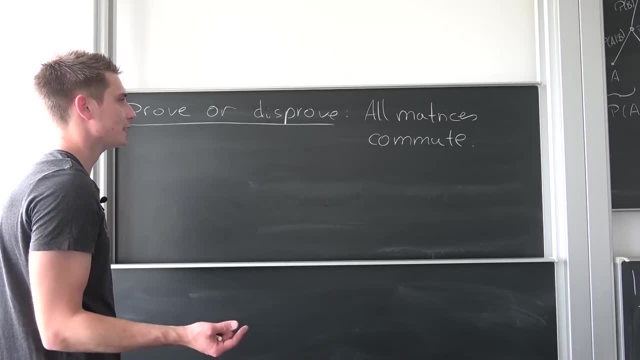 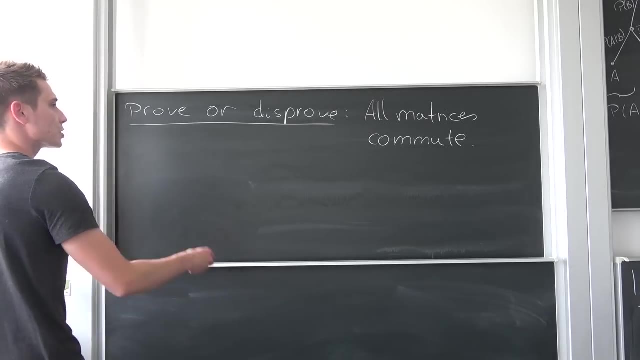 I think we are done, then I consider this to be proven Proof or disproof. All matrices commute. I mean if I just pick two matrices randomly, then that should definitely do the trick. I mean if it holds for one example, then it definitely holds for everything. So why not just pick completely random 0,, 1,. 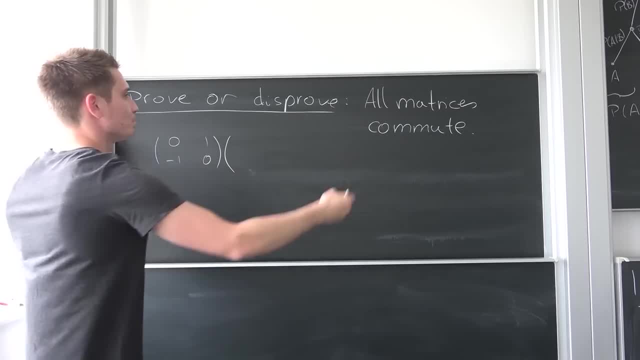 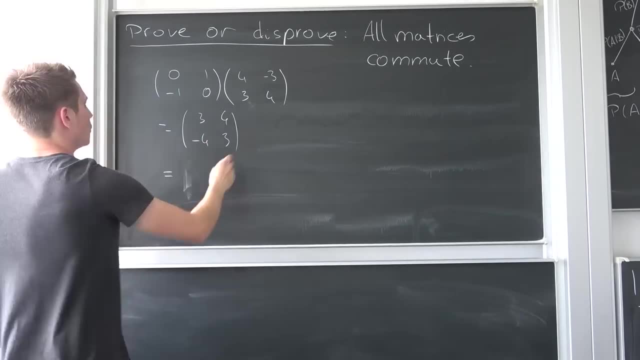 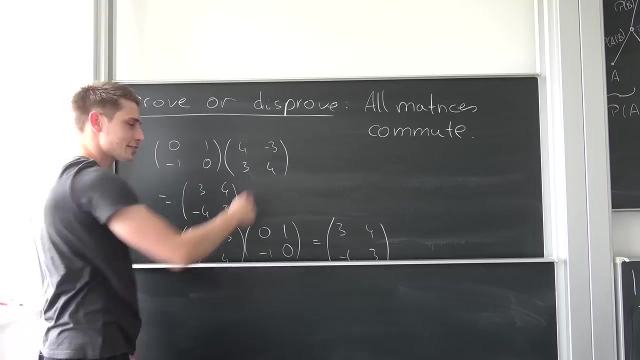 negative 1 and 0, and we are going to multiply it by I don't know 4, negative 3,, 3 and 4.. Hey, they actually commute. So that's definitely a true statement. That's so cool. That's so cool. 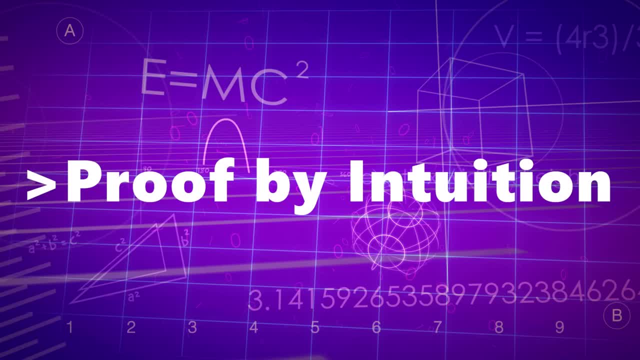 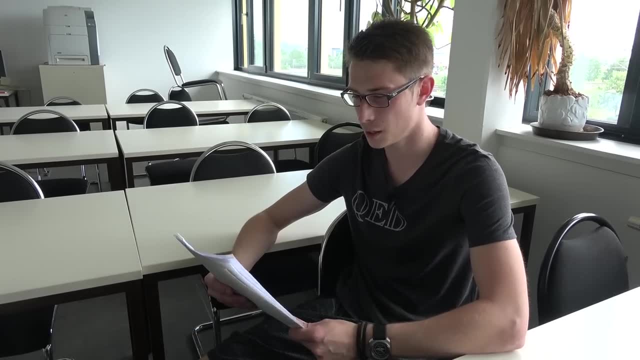 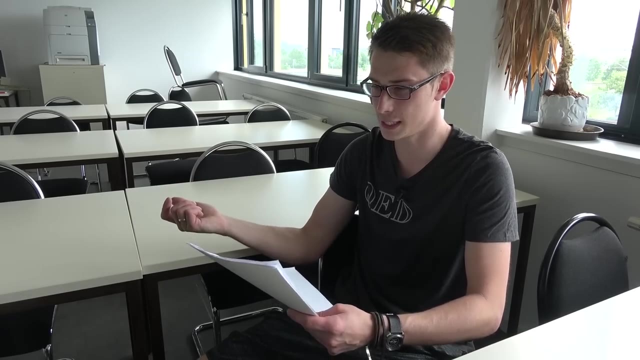 Okay. so what's on today's exercise sheet? Proof or disproof? The harmonic series converges. I mean it obviously converges because if we add smaller and smaller parts together, for sure it's not going to go to infinity. It's just like with the geometric series. 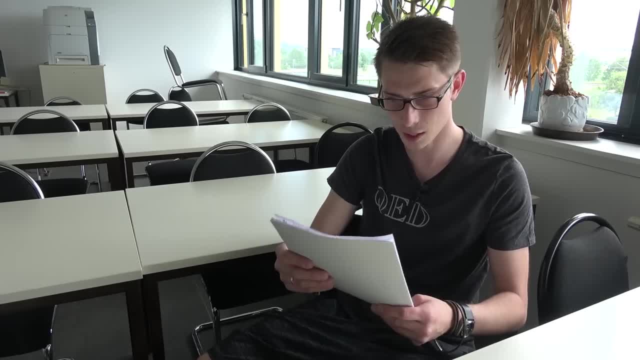 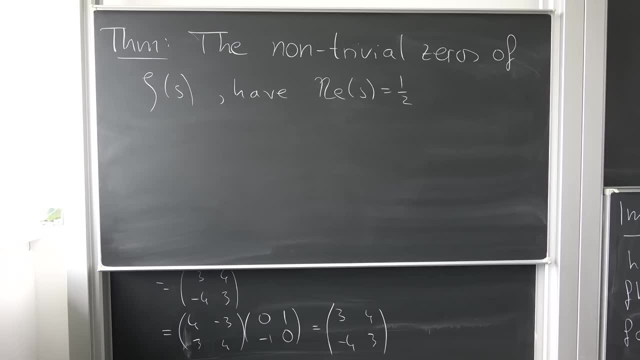 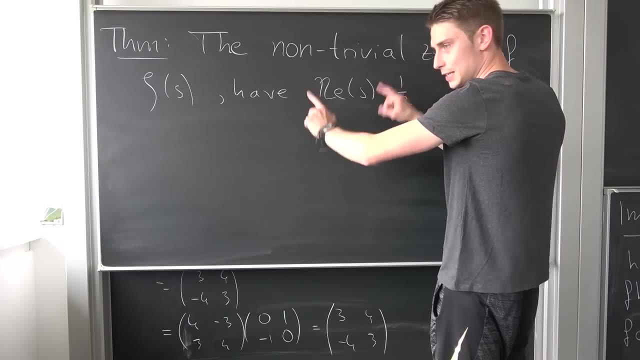 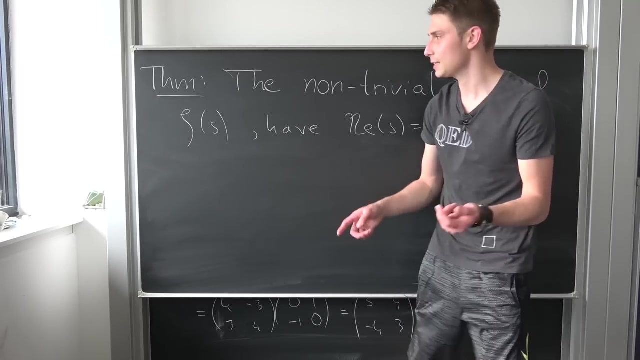 Yeah, okay, that's a nice intuitive explanation right here. I consider this to be proof, Jonathan, Jonathan, Big news. I think we finally figured this one right here out. There's such big news. Oh, really, Andrew, Yeah. so I asked professor Dodson and he said that this thing right here. 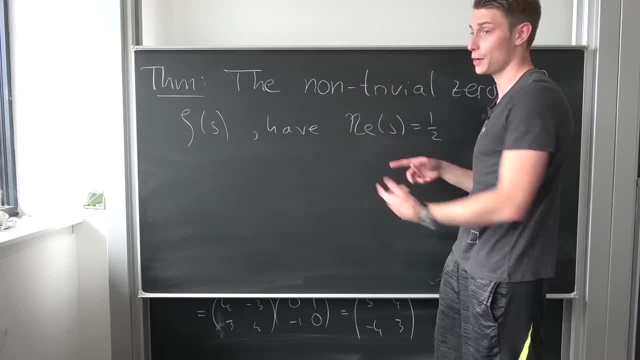 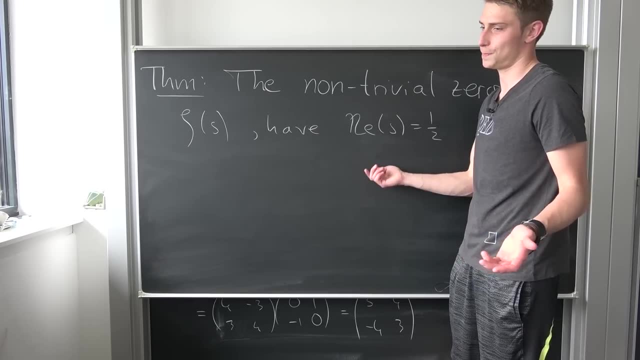 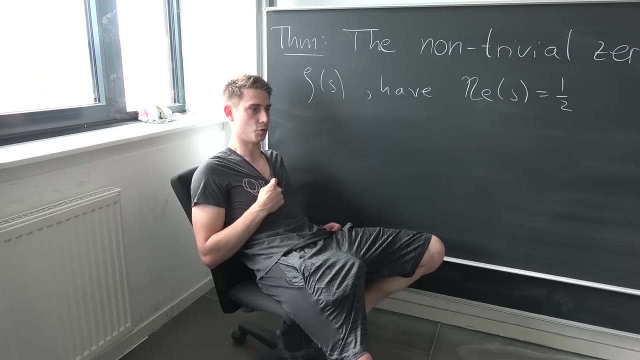 is probably true, Because a lot of It's probably true, because a lot of It's probably true, because a lot of proof theorems actually rely on this hypothesis being true. so I guess he's right. If professor Dodson says it's true, then it is probably true, For goodness. 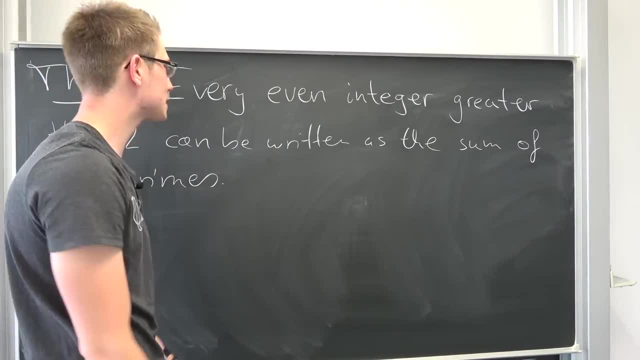 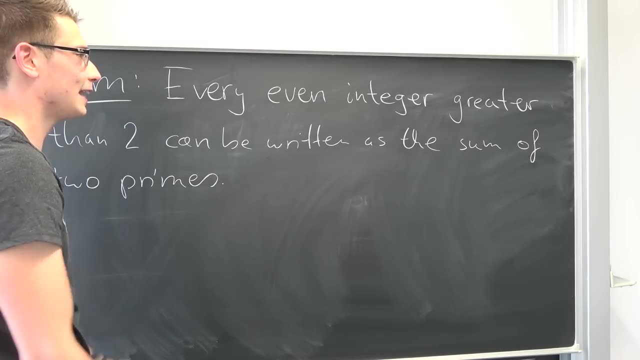 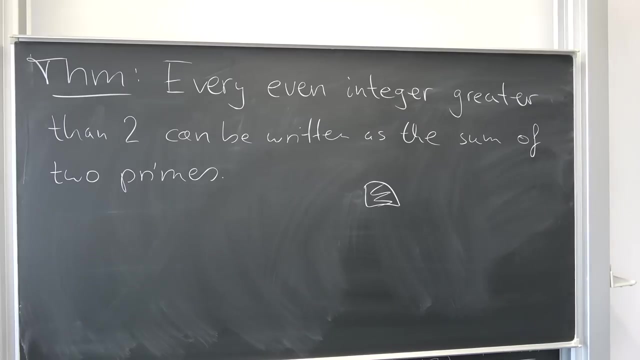 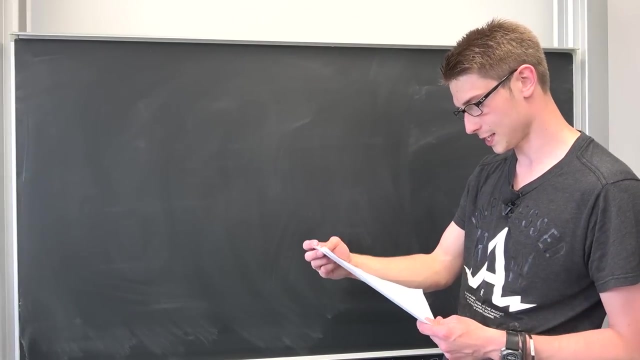 sake. I've been trying to solve this thing right here, to prove this statement, for five hours straight. why did mr Dodson even give us the stupid exercise? okay, I totally give up, I totally give up, I give up. oh boy, okay, Jonathan, last applied maths exercise for today. we have to show that sine of X is equal to X, for 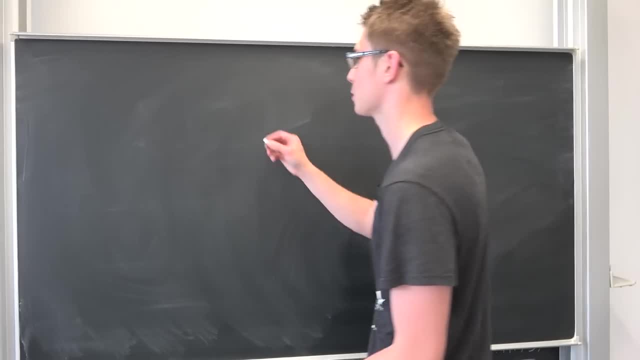 really small values of X. I mean, isn't that completely obvious if we just take a look at the graph right here? so that's a pretty good G-sign wave. if you asked me, it's a pretty good G-sign wave. if you asked me, it's a pretty good G-sign wave. 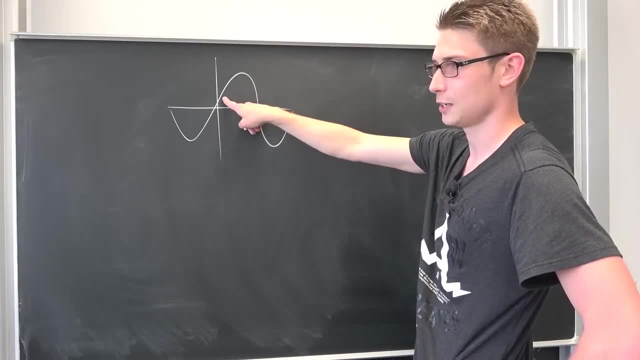 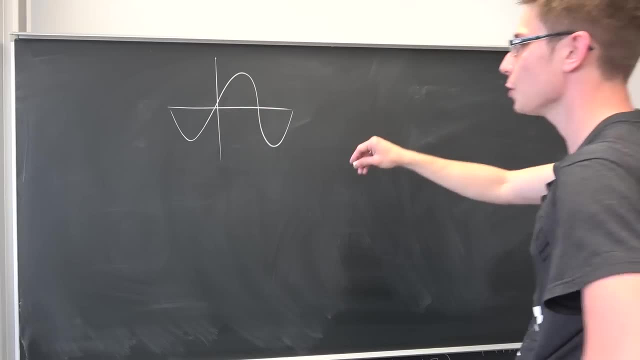 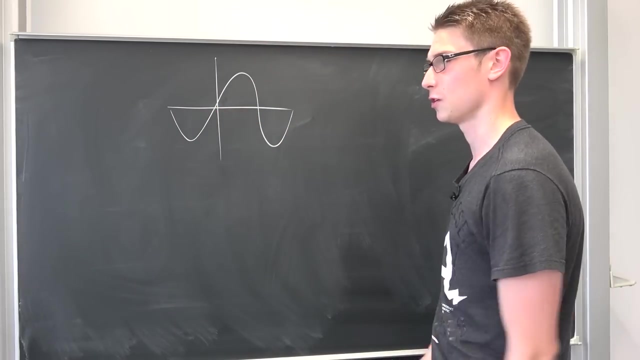 that's, it's quite a beautiful individual. yeah, obviously it holds right here, but in my opinion I- I mean, if you go way further and further- those lines come really close to the origin. so I don't understand why it's only for small values of X. is the sine of X, not X for every value of X? we have to ask the. 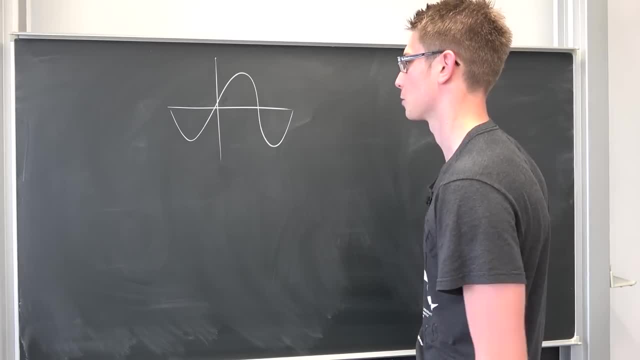 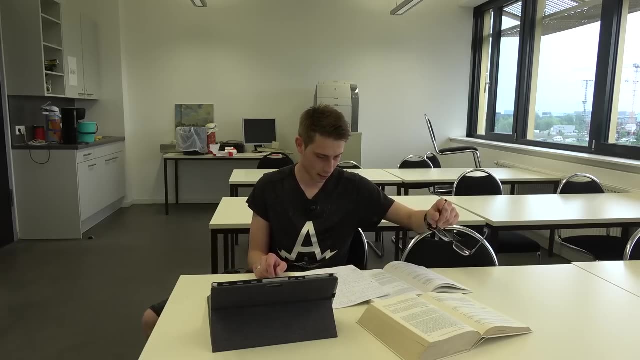 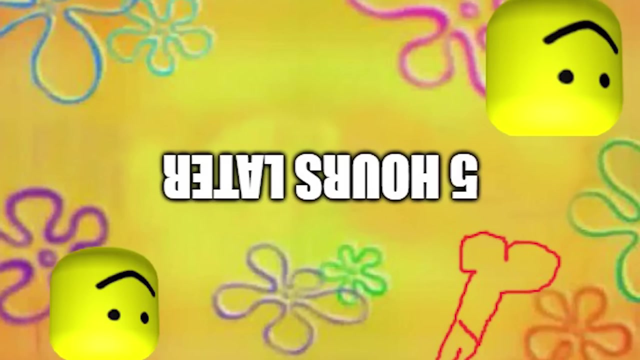 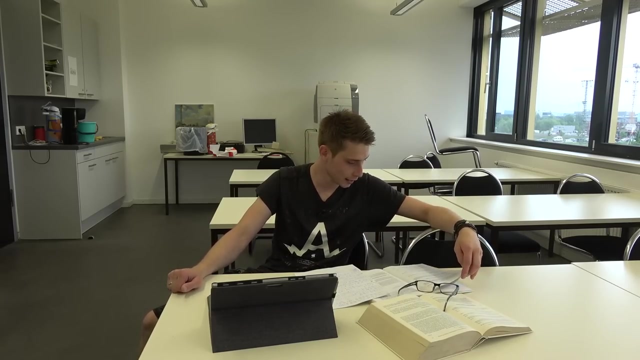 professor about that. I'm not really sure if he stated the theorem correctly. this last lemma, this bloody last lemma- it's the only thing stopping me from finishing up my PhD thesis. me, god damn it. this, this fucking thing, is unprovable. how should I even go about proving this thing? I have to do it. I just have to do. 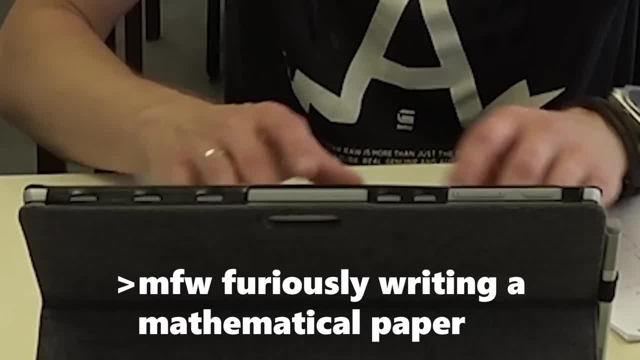 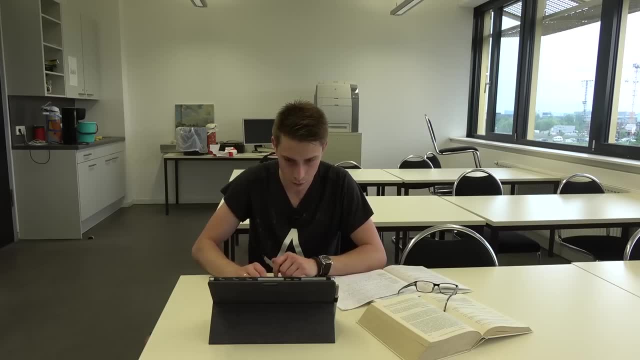 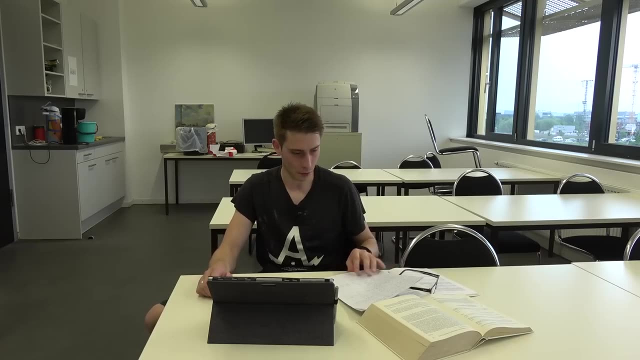 it and we are done okay, so I've written the paper. now I've included the lemma I couldn't prove also in this paper. but since I can't prove it, I'm just going to reference it and say that I have proven it in my PhD thesis, which I 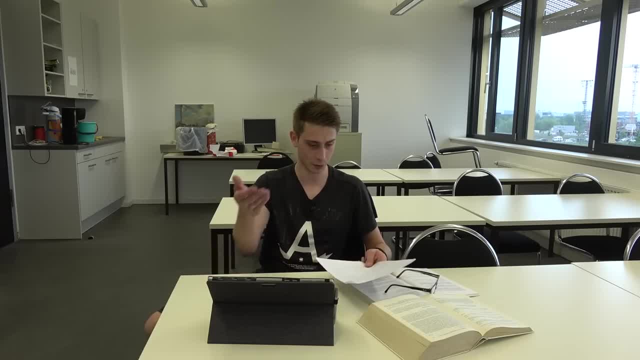 didn't. but no one's ever going to notice- because I'm going to reference in my PhD thesis- that I proved this very lemma that I couldn't prove in this paper that I'm going to publish to the Mathematica Society. so that's going to work wonders. no one's ever going to notice that. I have no idea how to prove. 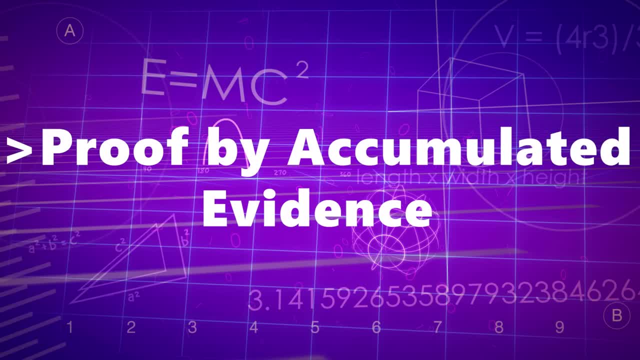 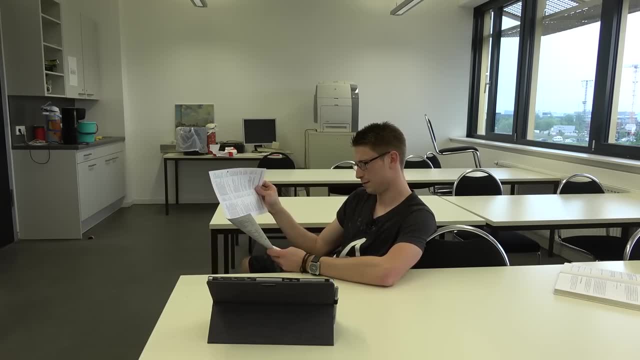 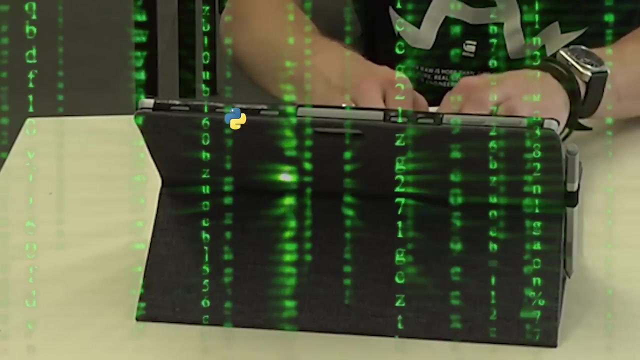 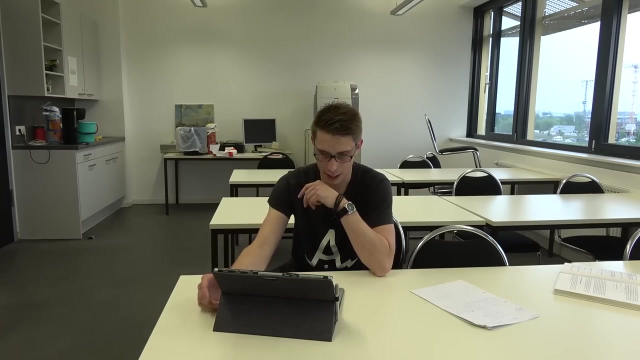 this thing so genius, it's so genius. okay, exercise number nine. it what it says, something about the Collatz conjecture that we have to prove, whatever the fuck that is. it seems like I could actually prove it numerically, okay. so what does Python say? I've checked the first 10 million numbers and